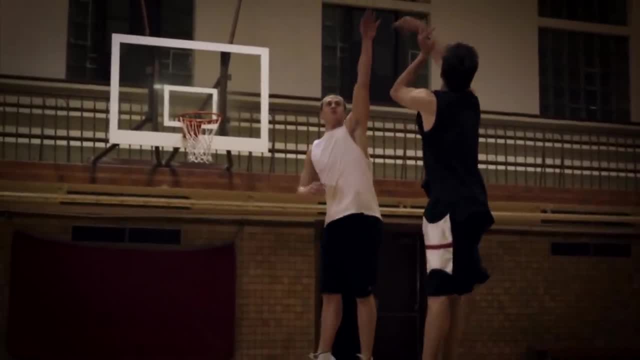 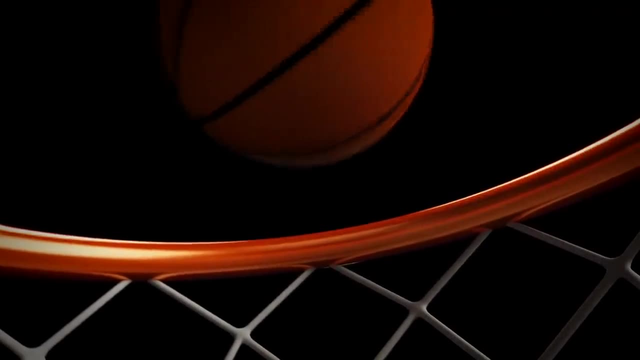 If we know the position and motion of a basketball at one instant and all the forces that act on it, we can work out from the classical laws of motion exactly where it will be at a later time. But quantum mechanics doesn't let us do that for a particle- All it tells. 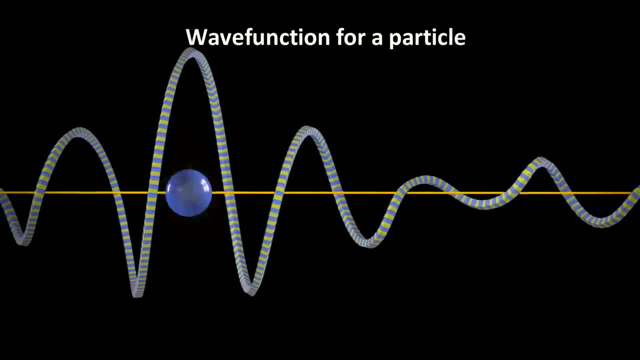 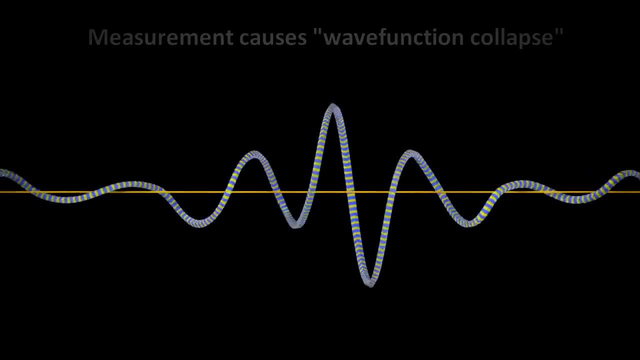 us is where the particle could be at the later time and what's the probability we'll find it there. So how does the indeterminate world of quantum mechanics, where the future isn't fixed, become the classical world we experience, where at least some things are predictable? 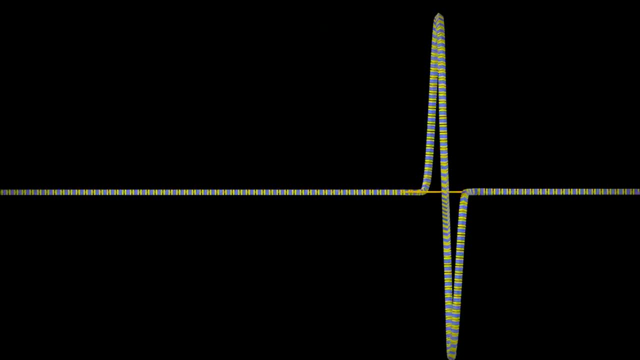 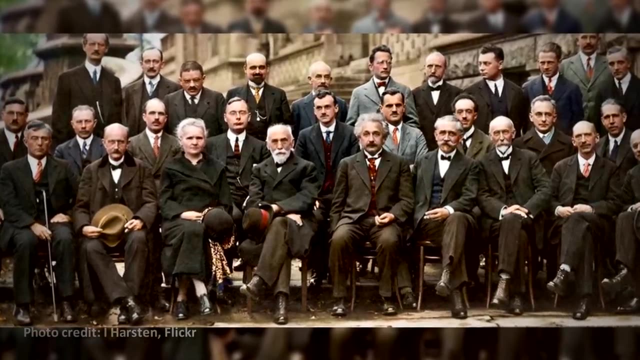 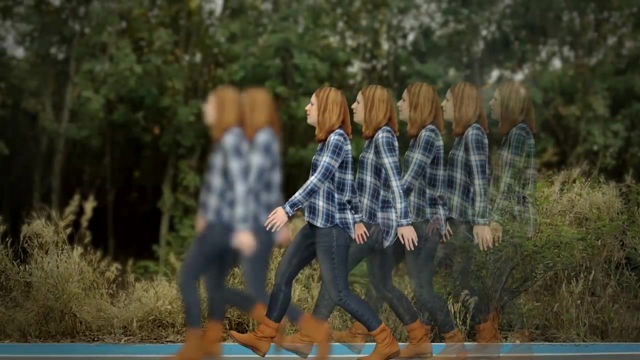 There's a traditional answer to that, but we now know that it's not a very good answer. In fact, quantum researchers have been arguing about it ever since quantum mechanics was invented in the early 20th century. I'm going to tell you the new story, or at least as much of it as we now understand. 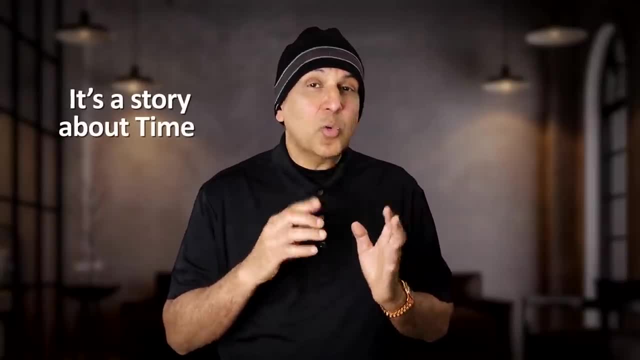 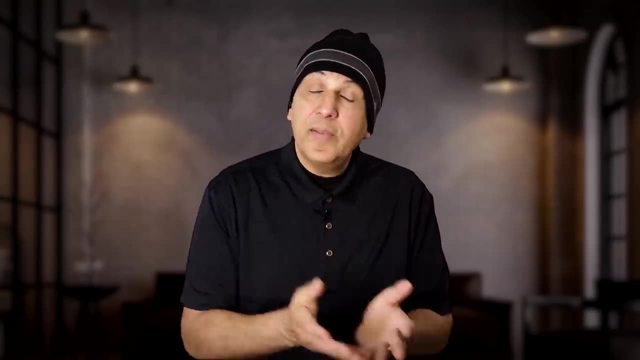 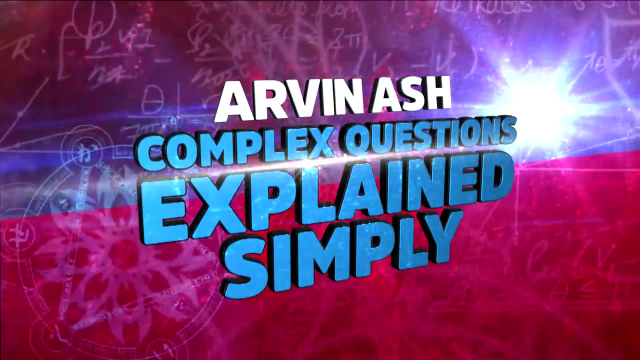 And, at its essence, it's really a story about time and the boundary between becoming and never-ending, Between the possible and the actual, And that's coming up right now. First, let me explain what I mean about the quantum world being indeterminate. 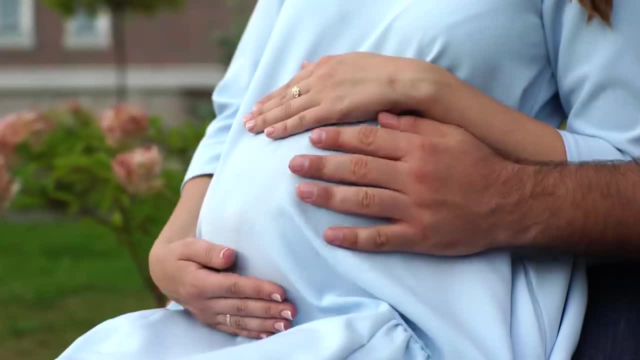 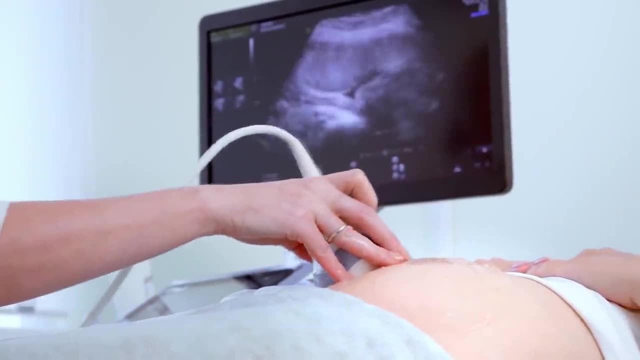 When a woman is pregnant, she and her partner can choose to know in advance whether the baby is a boy or a girl, or they can wait for the surprise at birth. All they need is an ultrasound scan. Once you look, you know. But if you don't look, you don't know. 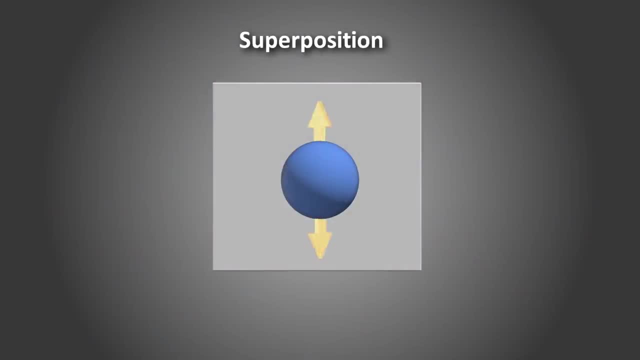 Now imagine a quantum particle that has been put in a state where, if we look at it, we might find, with 50-50 probability, that it's either this or that, Not a male or female particle, of course, but we might find it spinning, either one way or the other, which? 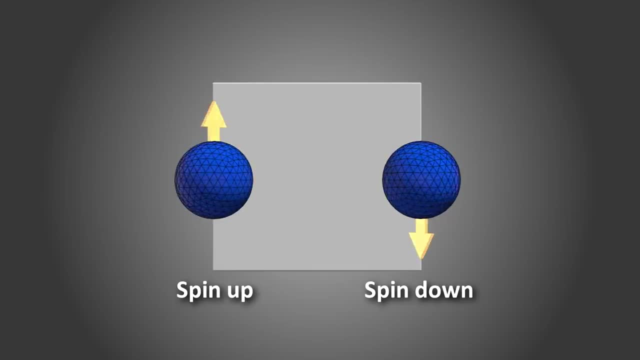 physicists call spin up or spin down. You might think that here too, the particle is always definitely one or the other, that we'll just find out which it is by looking, by making a measurement. But that's not the case. Quantum mechanics is not just about measuring Quantum. 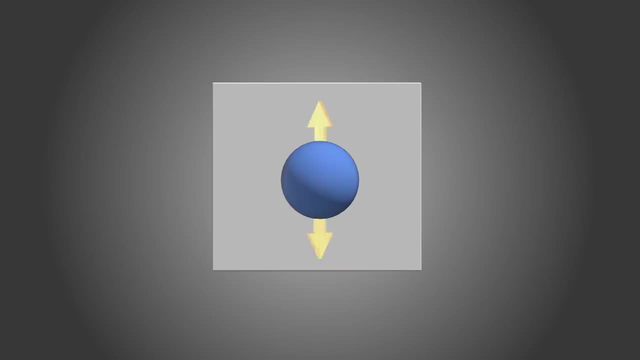 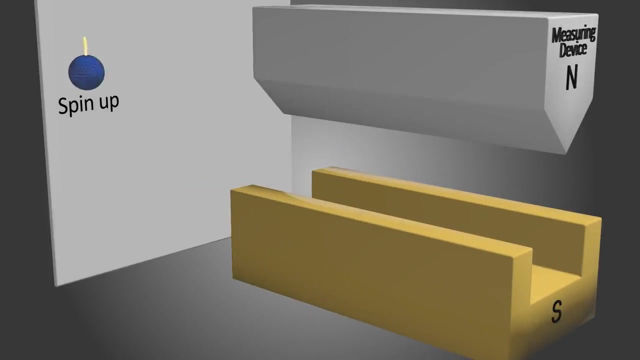 mechanics seems to insist that the spin has neither one direction nor the other. until we look, until we measure it, The very act of measuring forces the universe to make that choice. If the classical world was like this, it would be as though the baby is neither male nor 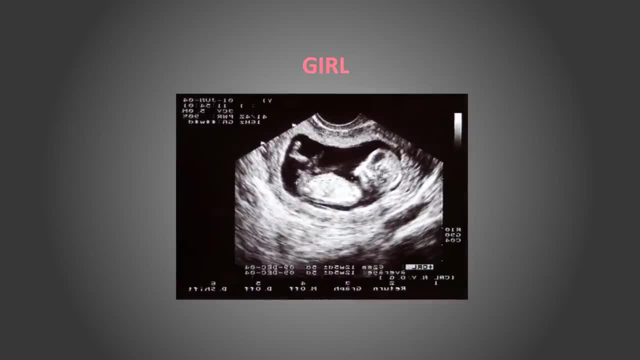 female, until we perform the ultrasound, until we look, Then before we look, we'd have to say that the chances are 50-50,. not because we don't know the answer, not because of ignorance, but because there genuinely is no answer. 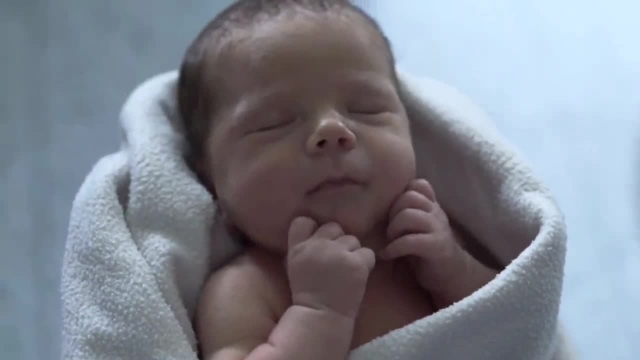 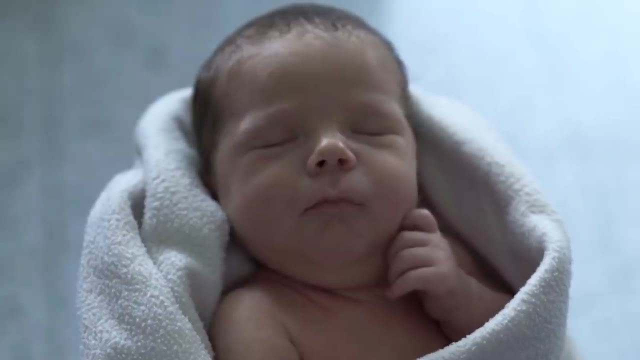 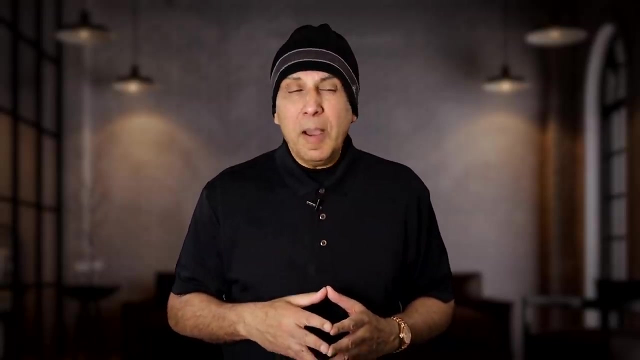 There are just probabilities. When we look, the probability then seems to switch abruptly from 50-50 to 100-0,. one way or the other, The baby becomes definitely a boy or a girl. This sounds nonsensical for a baby, but it's precisely how it is for a particle. 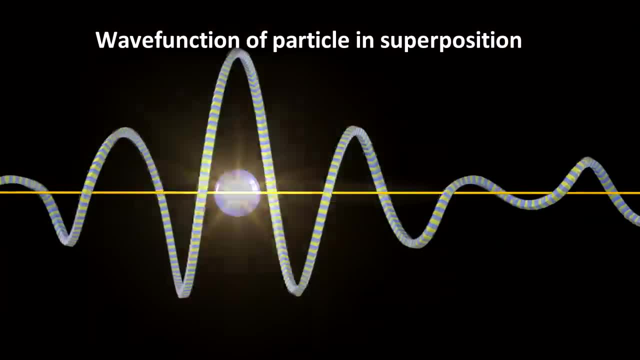 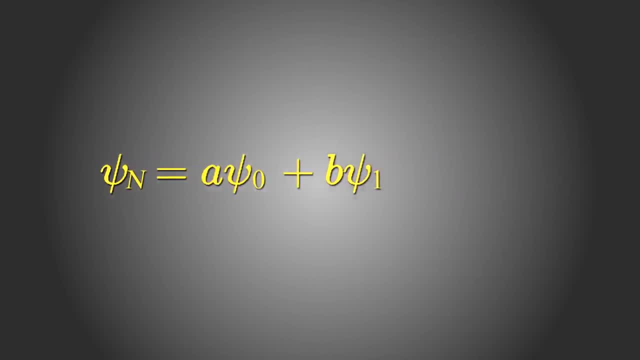 Particles are in what's called a superposition prior to measurement. What does this mean? All the variables that characterize the properties of elementary particles, such as its position and momentum, are encoded in a mathematical expression called a wavefunction, And while the particle isn't measured, the wavefunction is just the sum of all the wavefunctions of 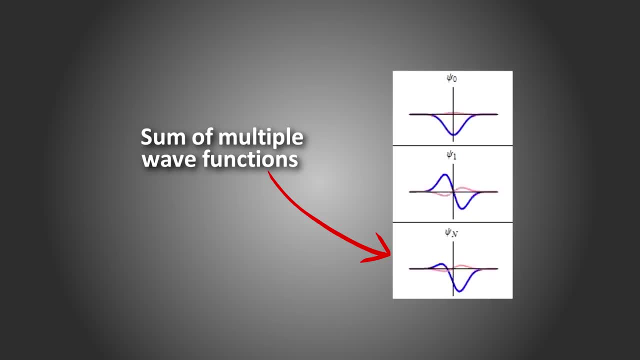 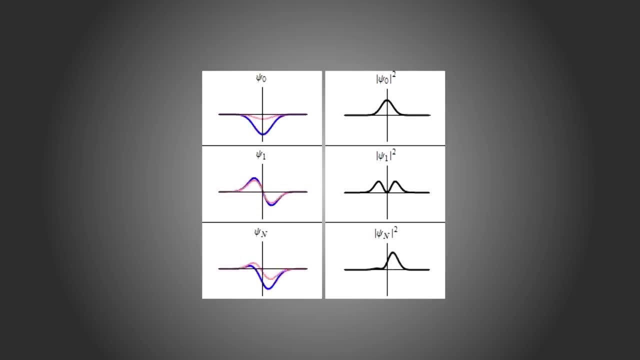 the states that the particle could be found in. This is called a superposition. By itself, the wavefunction doesn't have any intuitive meaning, But the square of the wavefunction gives us the probability of finding that quantum object in any particular place. 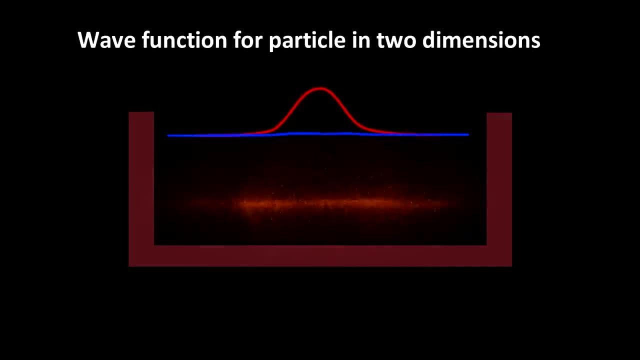 The picture seemingly makes no sense from a classical perspective because if we look at it, it looks as though before a measurement, the particle must be in all those places and states at once, And although I myself am guilty of characterizing it that way, that's. 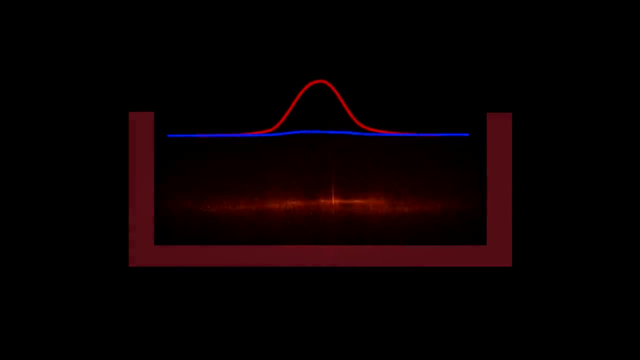 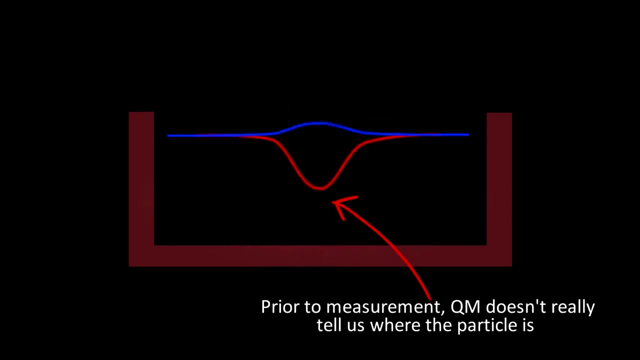 probably not what's happening Prior to measurement. quantum mechanics doesn't actually tell us where the particle is or what it's like at all. It just tells us the chances of what we'll see if we measure it, if we look. So now you might ask: how do we know? 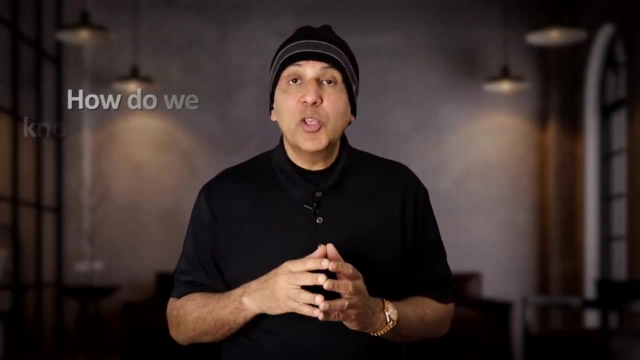 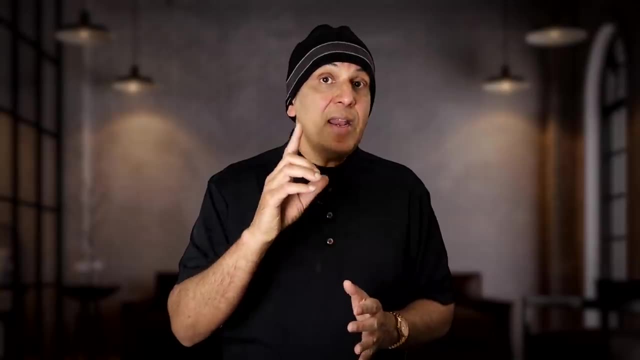 what's really true if we only see just one value of those variables when we look, We know it because even though those superposed states cannot be observed directly, they can and do interfere with each other, In this famous double-slit experiment, for example. 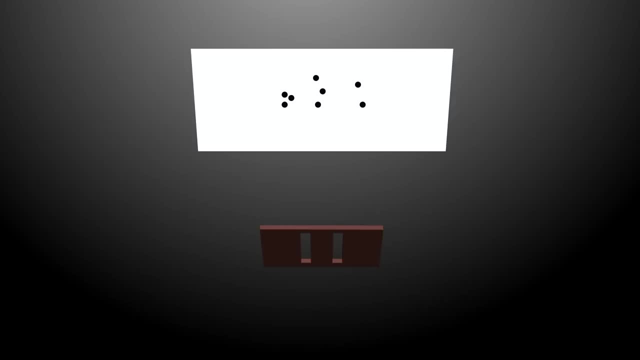 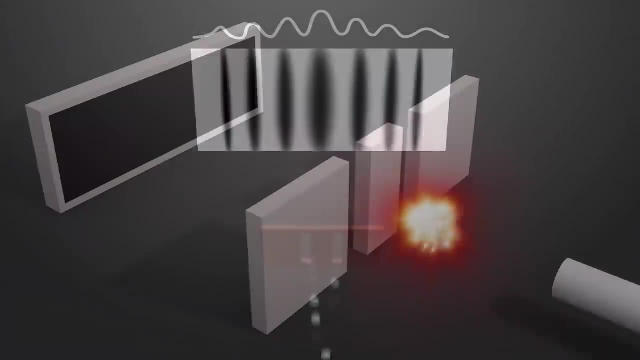 where particles like electrons are fired at two slits in a screen, we see an interference pattern on the far side, caused even by electrons fired one at a time. It's as if each of them goes through both slits for the same spot, making the difference. That's not true now. 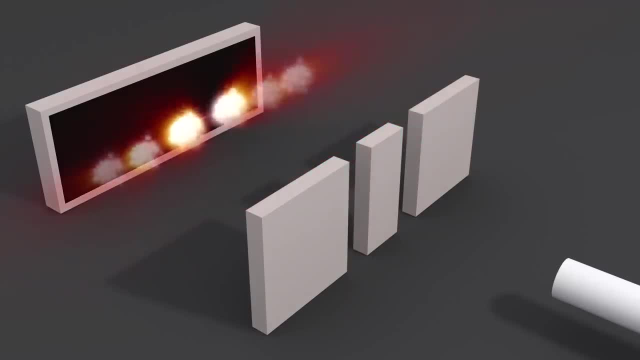 We only see those superposites, but actually in our experiment they're not superposites. slits at once and interferes with itself. These superpositions and the interference they cause can only persist as long as we don't try to find out where the particle. 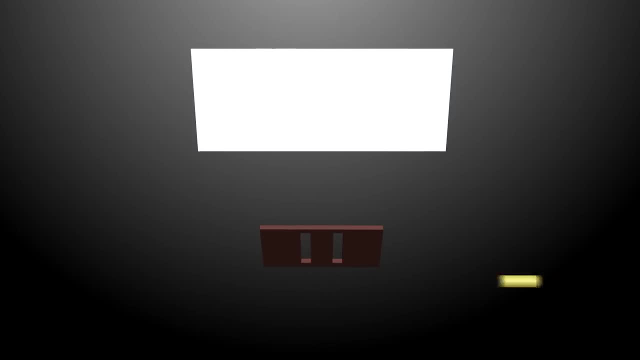 actually is or what state it's actually in. If we do, these quantum effects vanish and the particle becomes like a classical object with definite positioning properties. And that's the real problem. Quantum theory doesn't tell us how the switch from probabilities to certainties happens. All quantum mechanics can do is describe the particle before we. 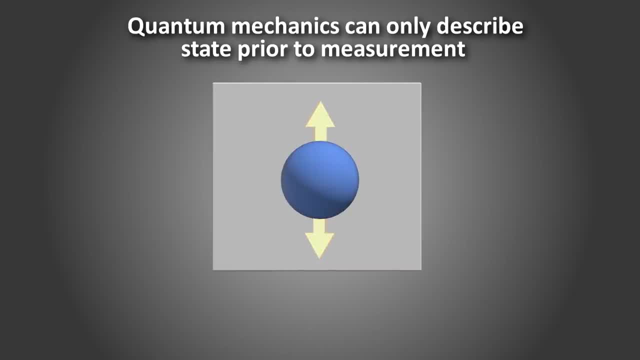 do the measurement when the chances of being spin up or spin down are, say, 50-50, or some other set of probabilities? According to quantum mechanics, there's no way a particle's wavefunction can abruptly switch from the 50-50 probabilities to the 100% certainty. 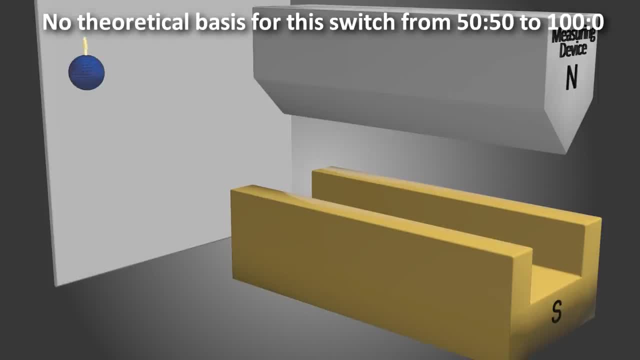 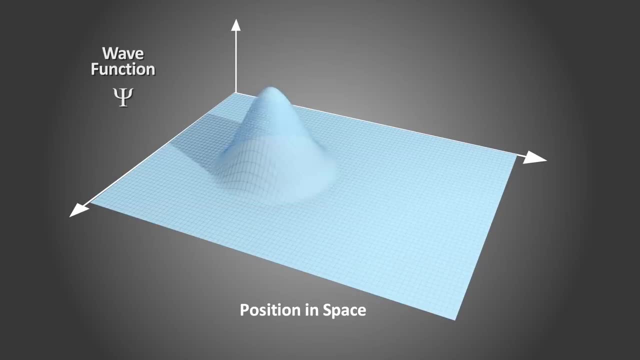 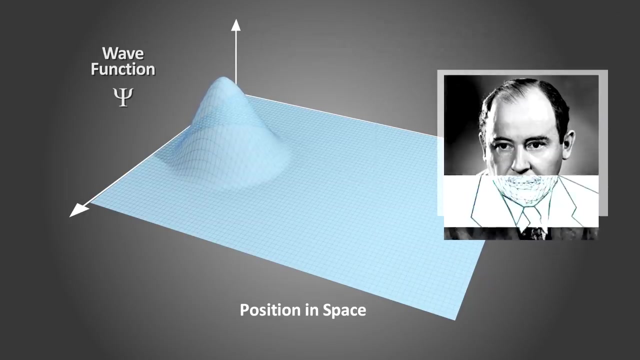 we get when we make the measurement. There's no theoretical basis for this switch, So quantum physicists have to add in that step by hand. This is something extra to quantum mechanics itself. This is often called the collapse of the wavefunction and was first introduced by the Hungarian mathematical physicist John 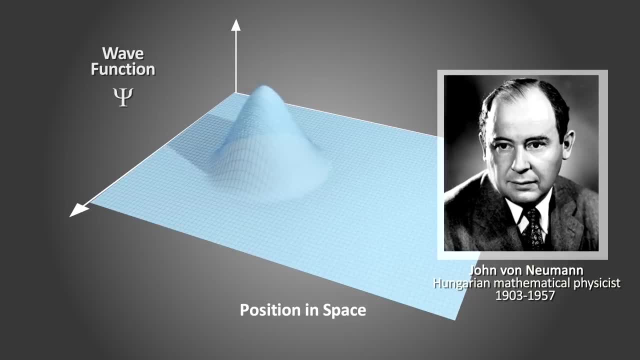 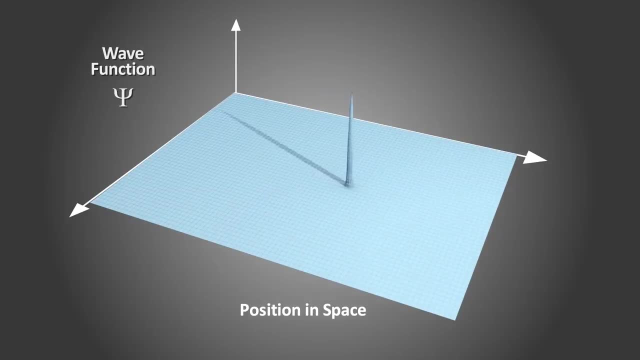 von Neumann in the early 1930s. But it's just a kind of botch for conjuring the classical world of this and that from the quantum world of everything-at-once probabilities. This is just not satisfying. In the past several decades, though, quantum researchers have realized: 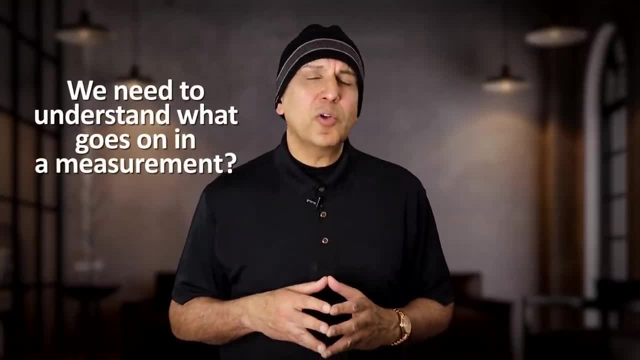 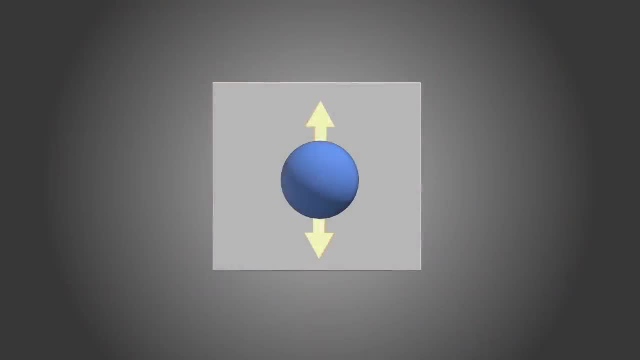 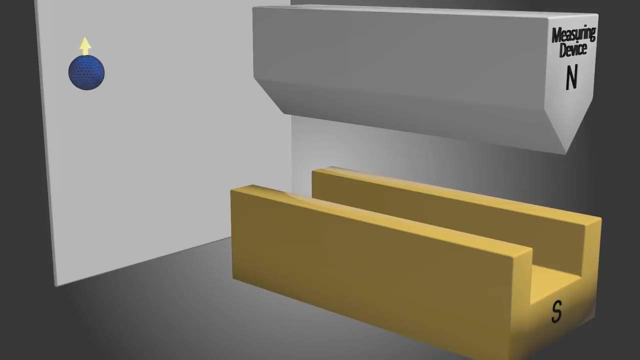 that what we really need to do to understand this thing we have called the collapse of the wavefunction is to think more carefully about what goes on in a measurement. It's not magic, after all. Whatever the quantum object is that we are measuring- let's say we are trying to find out the spin of that lone particle. we 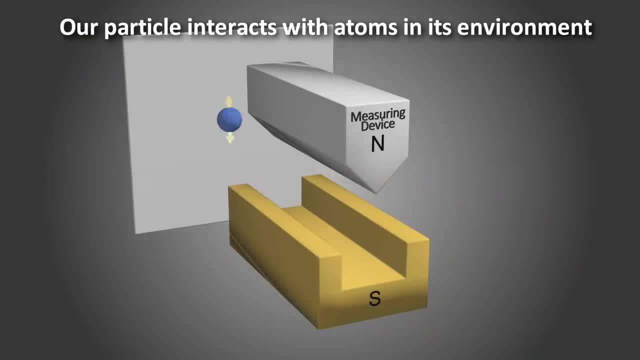 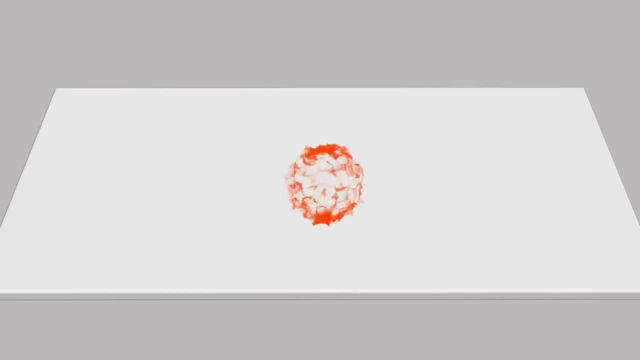 need some way of getting it to interact with atoms in its environment, especially those in our great big measuring device. According to quantum mechanics, what that means is that the quantum state that the particle is in becomes mixed up. The particle word is entangled with the states of the atoms in the environment. If the particle 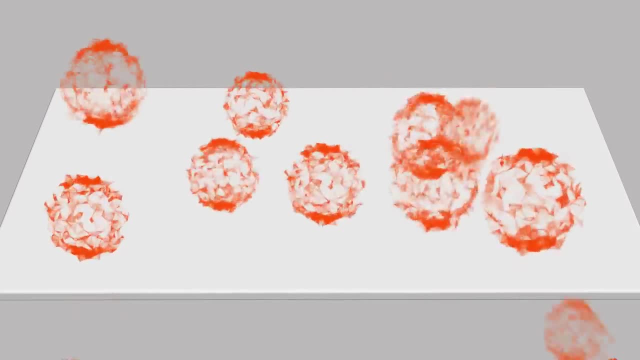 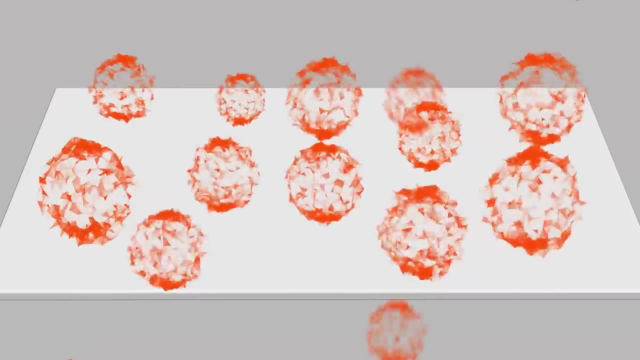 is in a superposition. this superposition then spreads to the atoms it interacts with. Through this process of entanglement, they all become part of one big superposition. It's one big entanglement party. The more of its environment, the particle interacts. 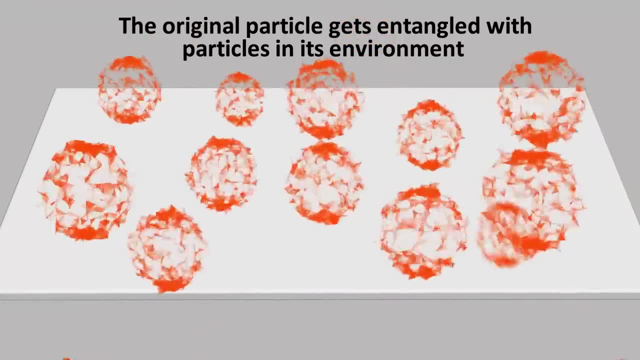 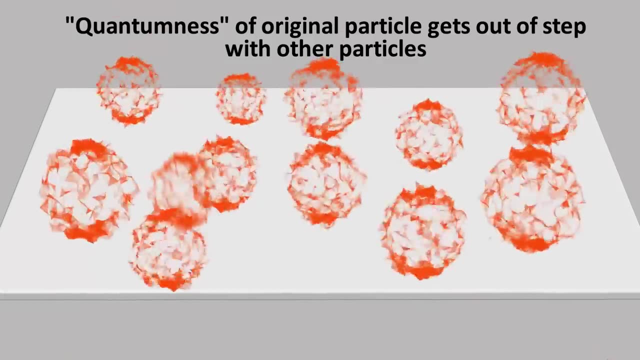 with the further the superposition spreads. So it's still a quantum system, it's still in a superposition, but it becomes everything Ever harder to see, in that huge crowd, any synchrony between the waviness of the original particle's superposed quantum states. 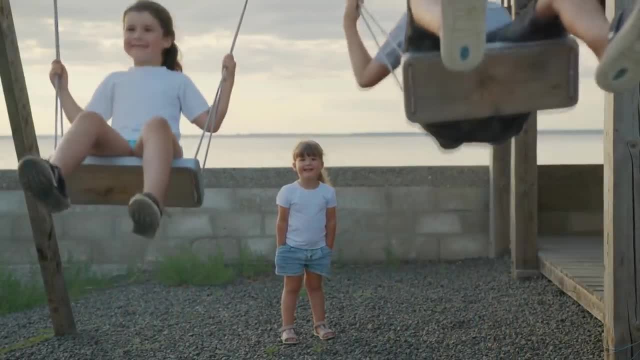 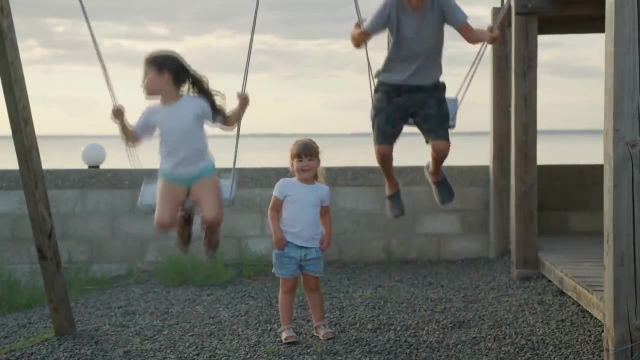 It's like a line of kids on swings. They might start off going back and forth in synchrony, but gradually that synchronization is lost. This is called decoherence. What you're left with looks like a mess of unrelated waves. If now you want to see the original. 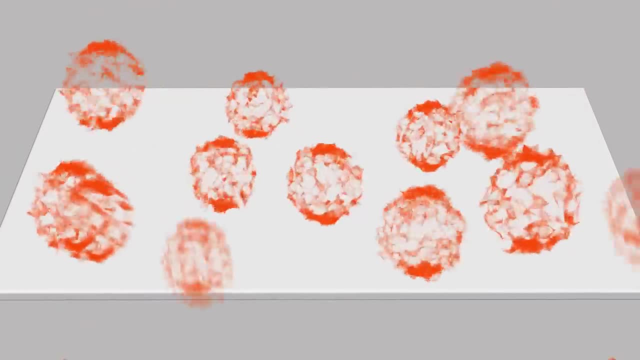 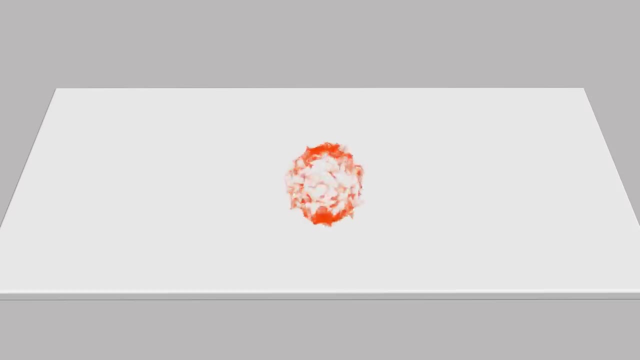 superposition. you would have to look at the quantum behavior of all those entangled atoms to get the full picture, But pretty quickly this becomes impossible. It's literally like trying to keep track of the effect a floating dust grain in the air has on all. 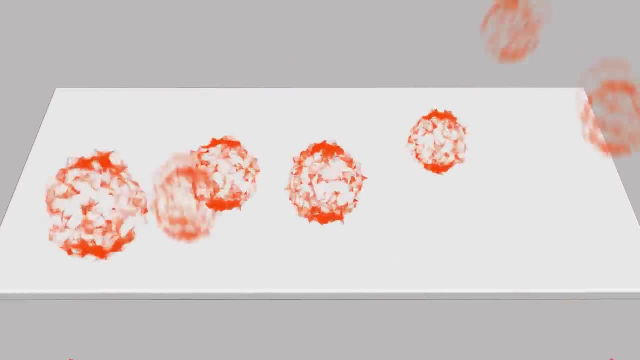 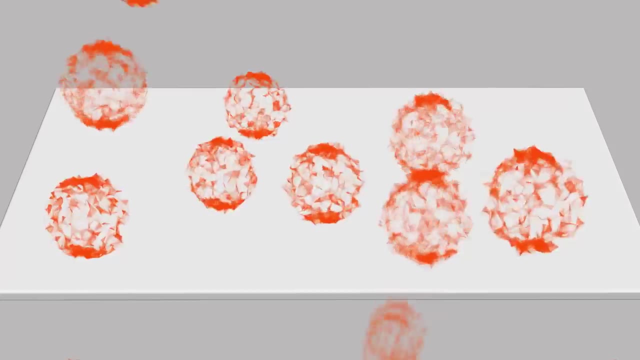 the atoms as they collide with it and then with each other. So the entanglement spreads. It inevitably leads to ever more decoherence. This, you might say, dilutes the quantumness, hiding the superposition from plain sight. You can't see it any longer. 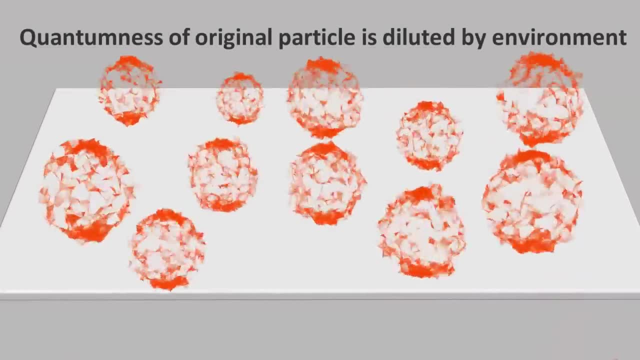 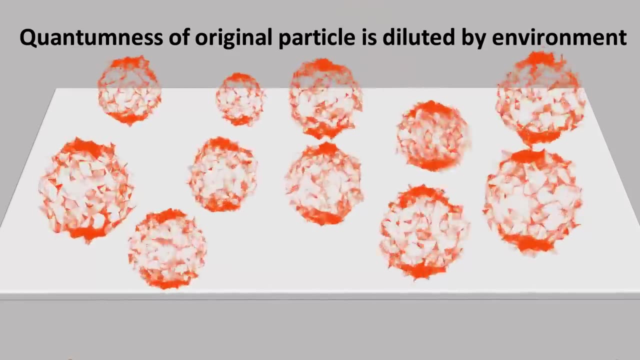 in the original particle. Instead, it turns out that the environment gets imprinted on it with the effects of just one or the other of the possible spin states selected at random, in much the same way that a needle on its tip will fall in one direction at random. 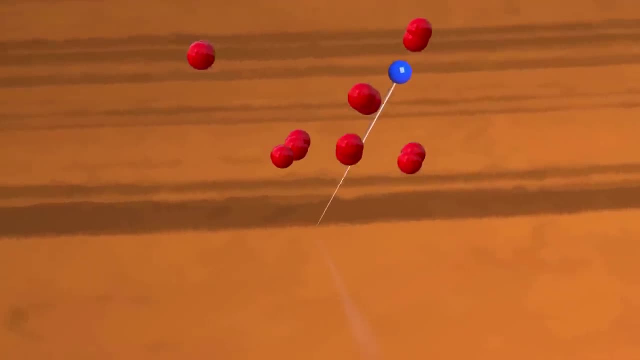 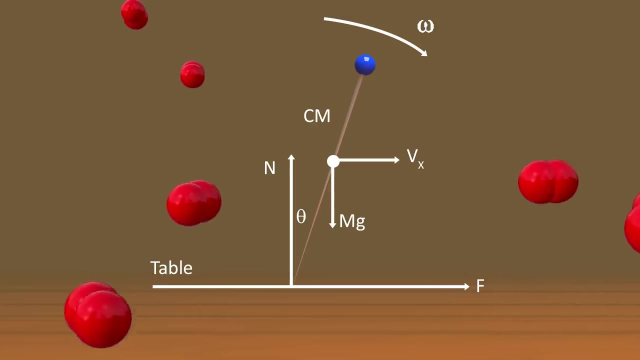 The difference is that where a needle falls is in theory predictable in advance if we know all the molecular interactions and forces acting on the needle. But this is not the case for our quantum object. We cannot know, even in principle, before it happens, which 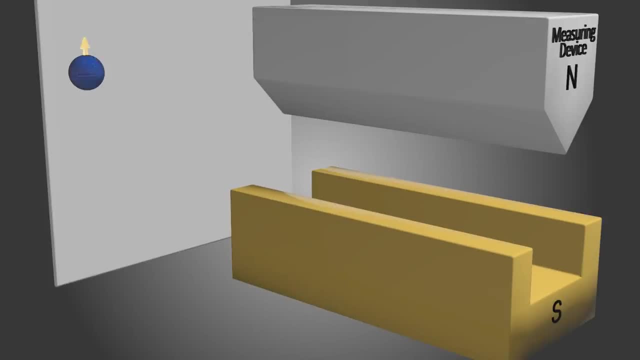 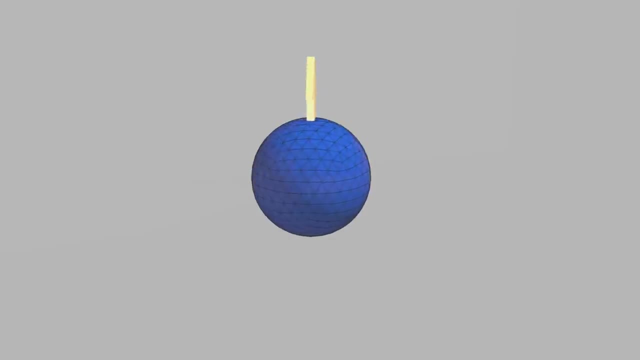 way, the decoherence will tip the balance. There's now a problem with the decoherence. It's not just a matter of whether or not it happens. We have a pretty good understanding of how decoherence happens and how it creates a classical outcome, a definite result from a quantum measurement. 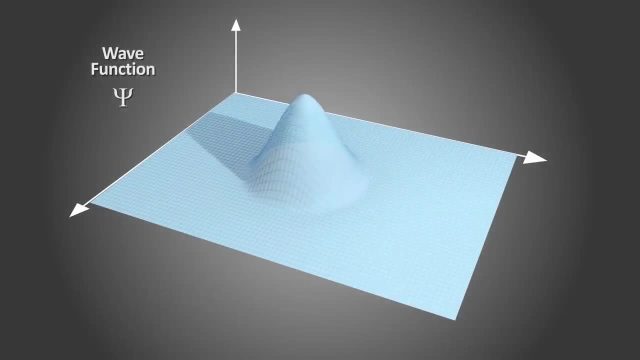 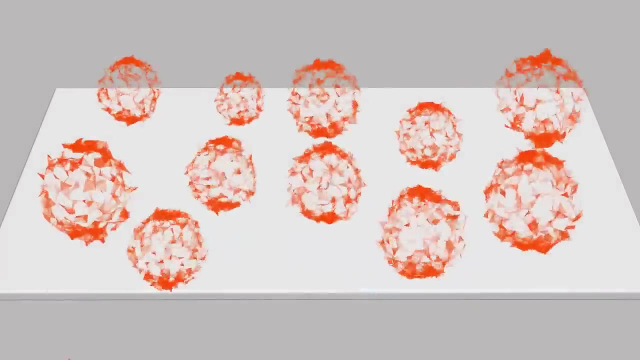 So, in place of the old sudden and slightly mysterious idea of wave function collapse, we now have a theory that, at least in some simple cases, can show us how decoherence produces classical from quantum. It's a real physical process and takes time, though usually a very 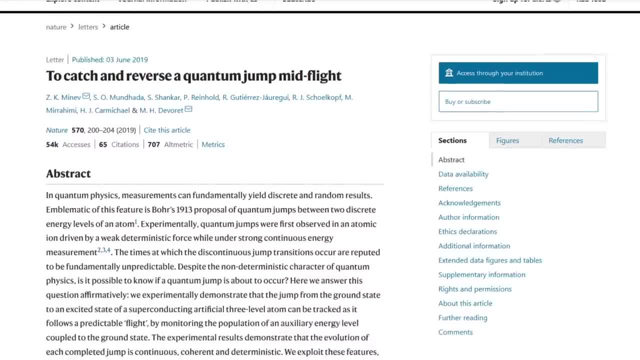 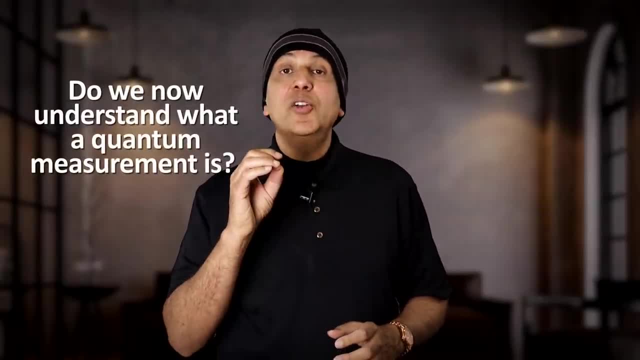 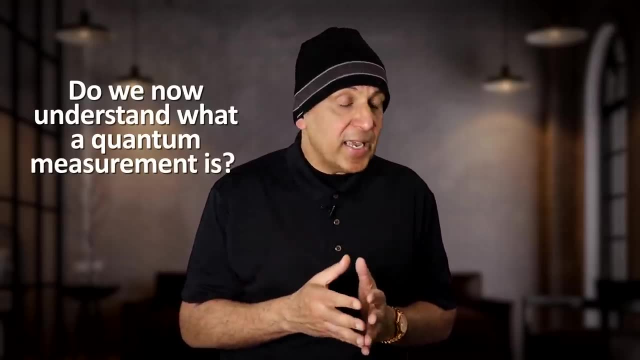 short time. Researchers at Yale University have even been able to track and record this so-called collapse process as it unfolds. Does this mean, then, that we now understand what quantum measurement is all about and that it's not really collapse at all, but just a gradual leaking and filtering of information? 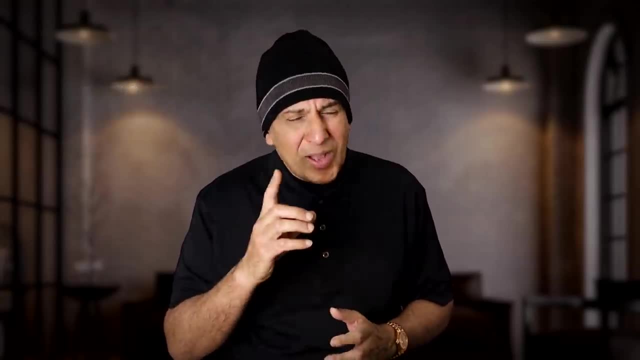 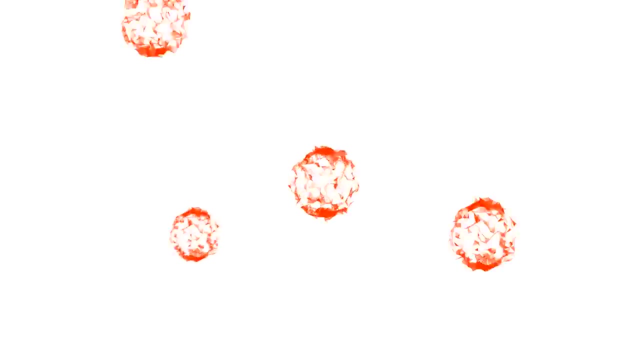 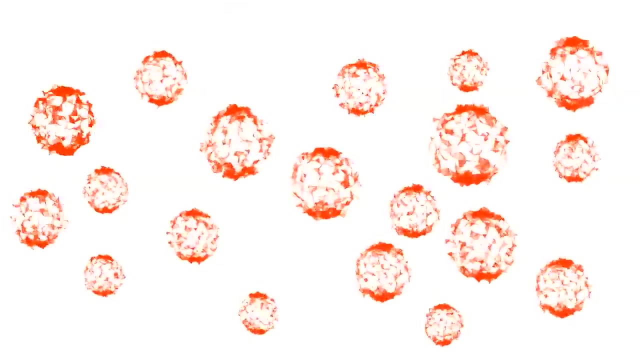 about the quantum object into the measuring apparatus. Well, not quite. There's a critical thing still missing, You see, as entanglement causes decoherence and spreads the quantumness only throughout the environment, there's no obvious end to that process. Every atom. 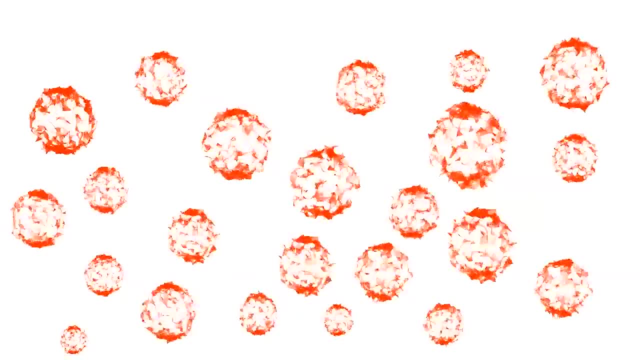 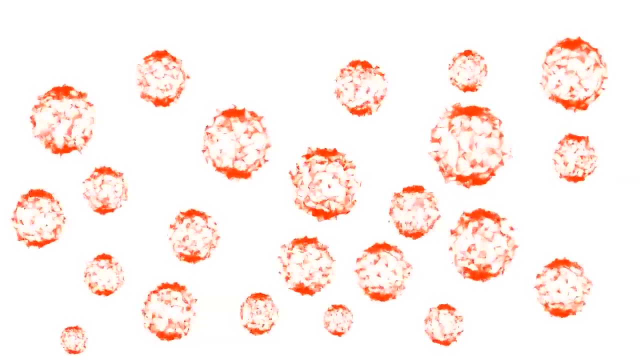 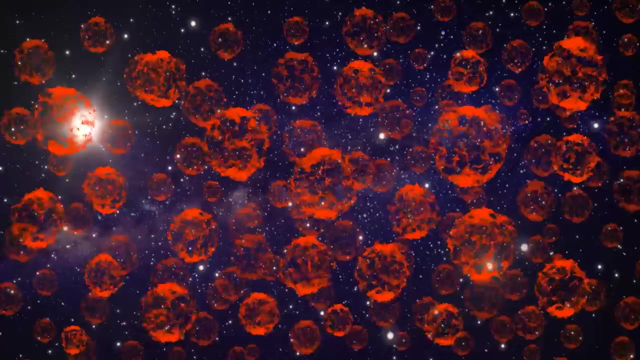 that interacts with an atom, that interacts with another atom, that interacts with the original quantum superposition, in effect gets tainted with a little bit of that superposition. It goes on and on spreading not only in the local environment of the quantum object but throughout the entire universe. This means that it very quickly becomes practically impossible. 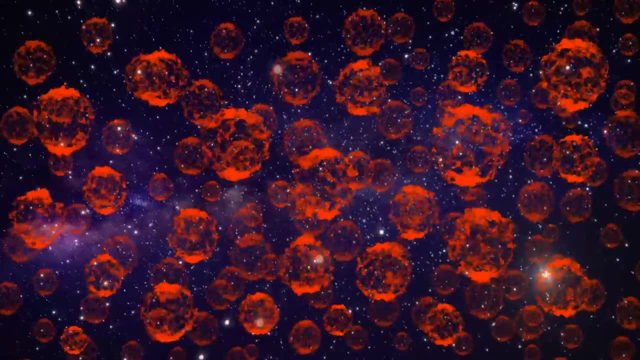 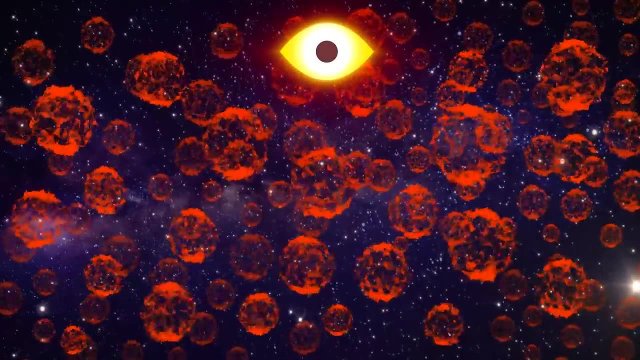 for us to keep track of, But there's no end to that. You can't really go beyond the track of how far the spreading goes and which atoms it entangles, But not in principle. If we were some god-like being that could watch every atom in the universe, then we 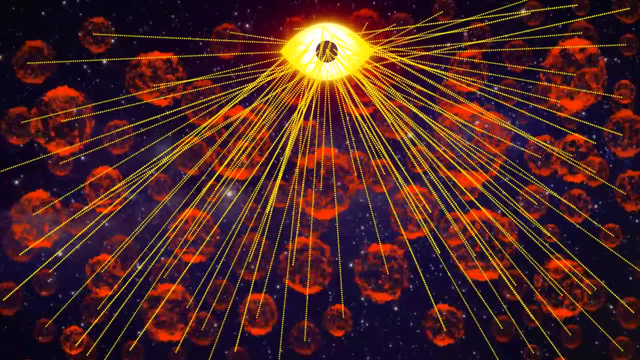 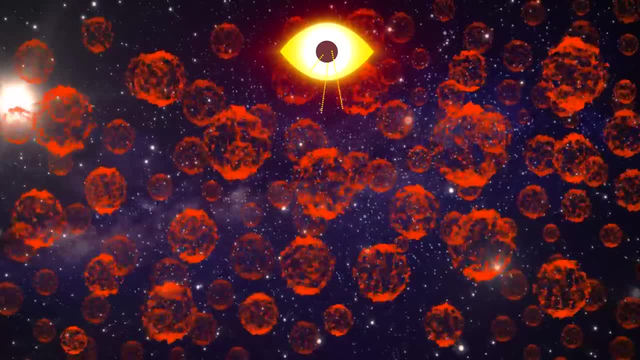 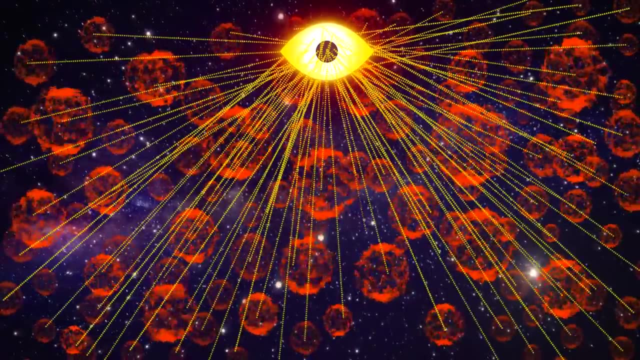 could at any moment identify all those that have become entangled by the act of measuring, of observing the original particle. If we only look at a few of them, we won't be able to see the entanglement, because decoherence has left their quantum waviness looking all jumbled and out of step. 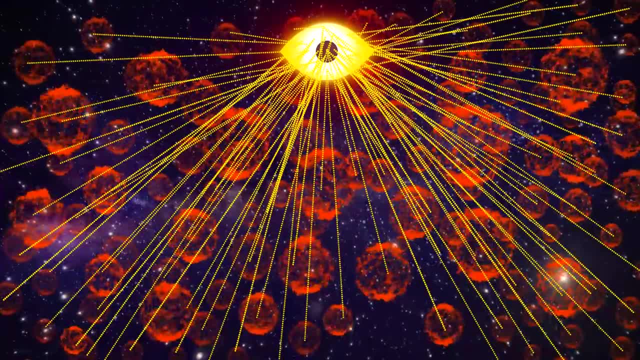 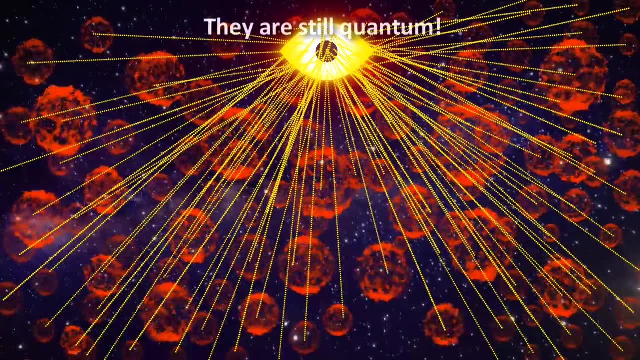 But if we could inspect all of them, we can make out the pattern and deduce that they are in fact all in a kind of massive entangled state of superposition. In other words, they're all still in a state of both this and that. 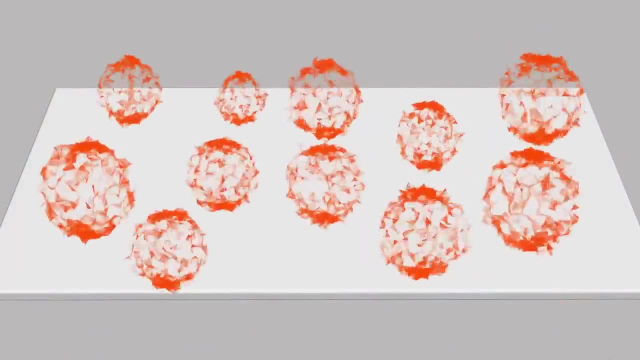 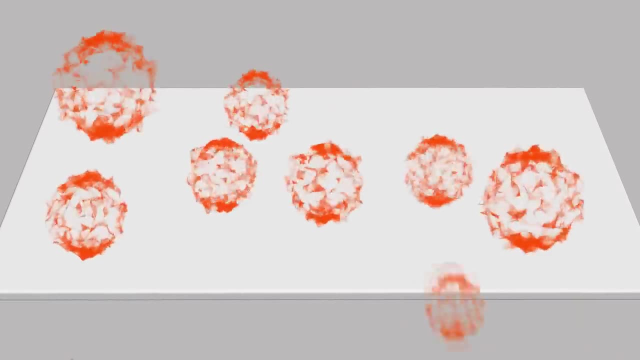 They're still quantum. What's more, it could be possible in principle to then reverse the whole process, to disentangle it all and focus all the quantumness back Into the original particle, recreating the superposition it started in. 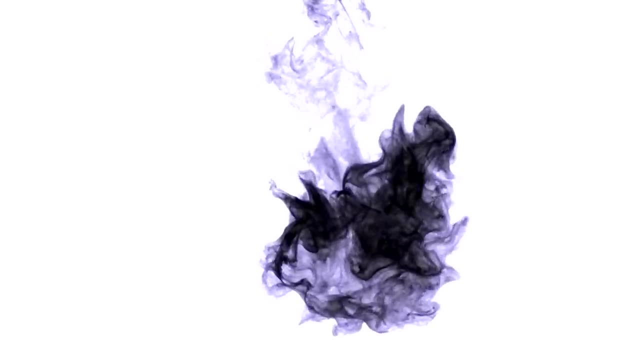 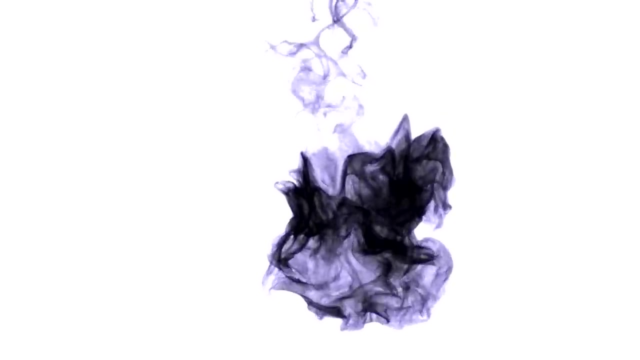 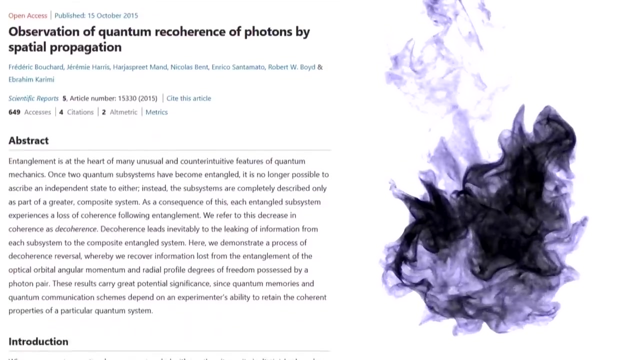 This would be like keeping track of every molecule in a drop of ink dispersing in water and carefully guiding it back to reconstitute the drop. It sounds absurdly hard, but actually there have been some experiments in which this sort of re-coherence has been possible for a quantum object interacting with just a few particles. 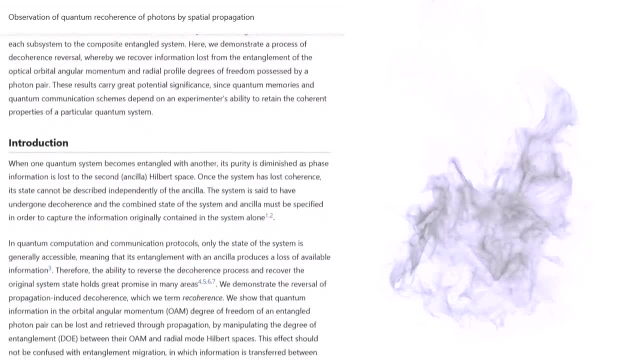 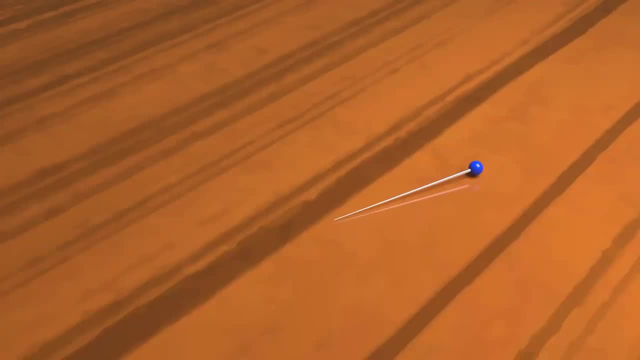 in its environment before decoherence has gone too far for any backtracking. That would mean undoing the measurement and erasing any information we gained from it, Forgetting where our needle pointed, Almost like reversing time itself. So here's the question. 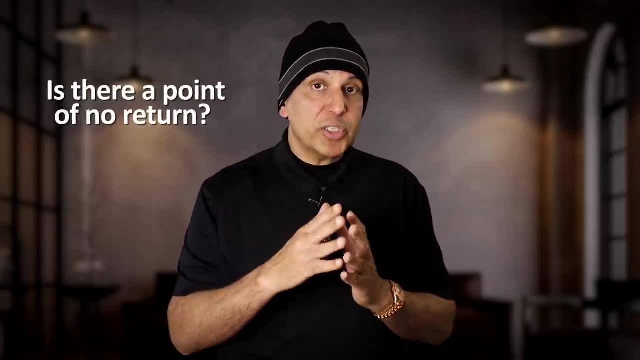 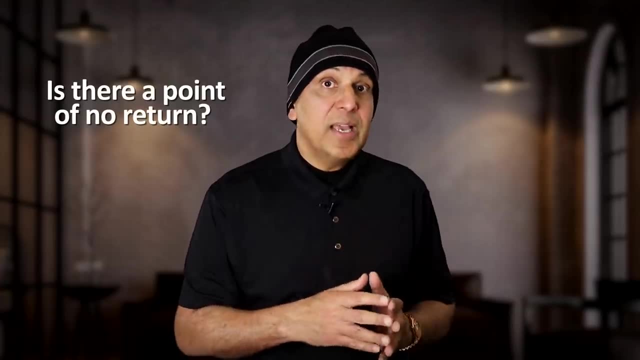 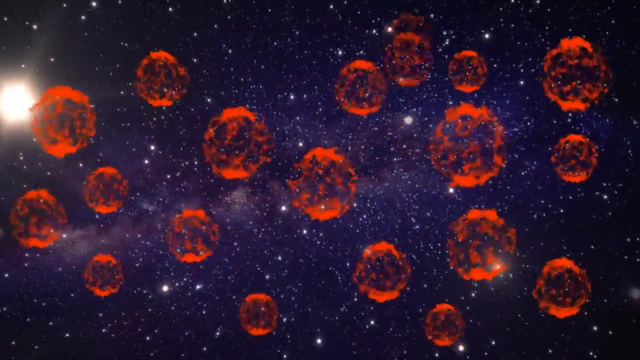 Is there ever a point where the measurement process switches from being fully reversible in principle by this sort of re-coherence and becomes irreversible? Is there a point of no return? Quantum experts don't agree about this. The theory that describes a measurement process as irreversible is the theory that describes 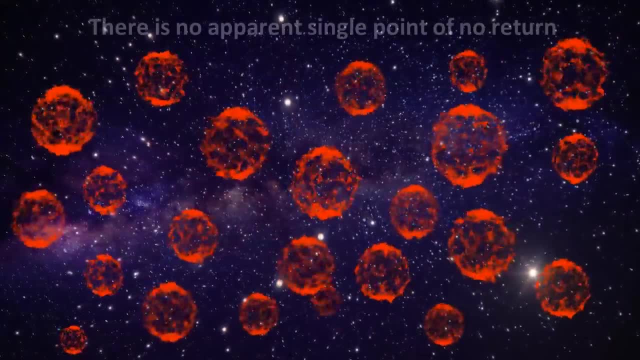 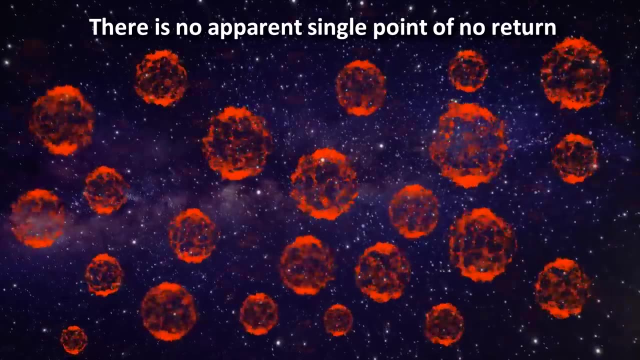 a measurement by decoherence and imprinting the result on the environment doesn't generate any such point of no return. But some believe that a point like that is needed to go from quantum to classical. As long as the process is reversible, it's still quantum. 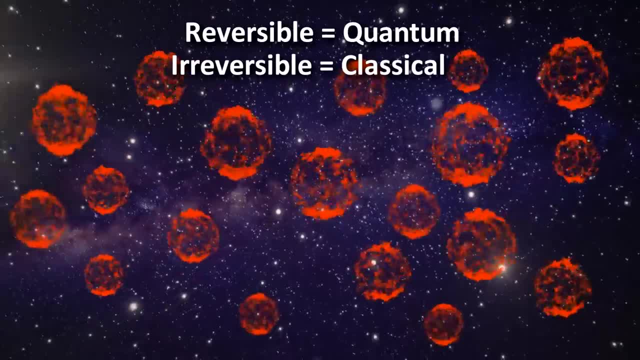 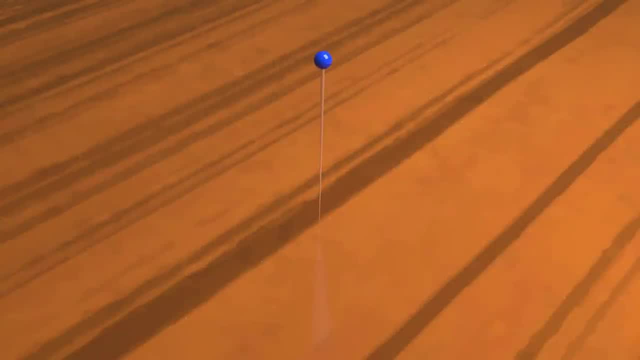 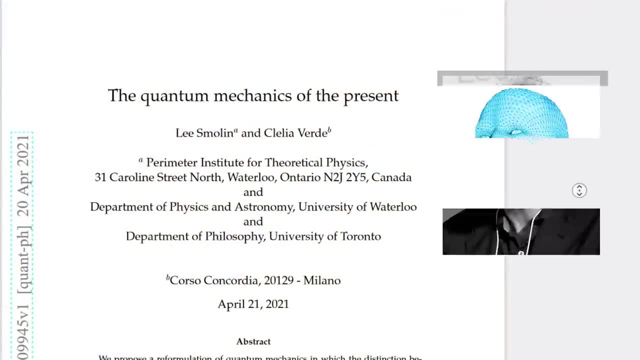 It's only when it becomes irreversible that it becomes classical, And it's only then that we can truly say what happened, which way the needle pointed, what the outcome was. In other words, It's only then that an outcome is real. Physicist Lee Smolin has recently suggested that this is in fact what distinguishes the 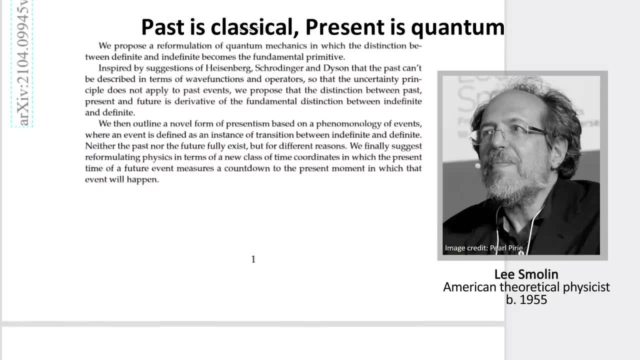 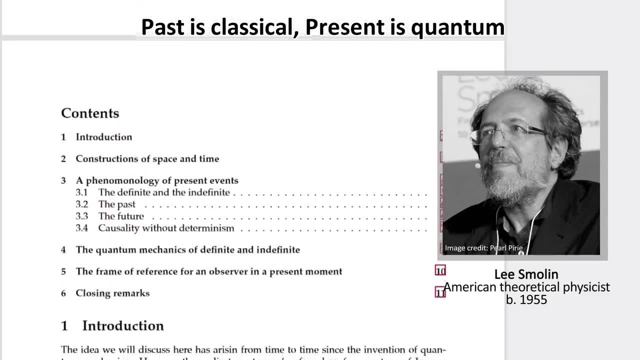 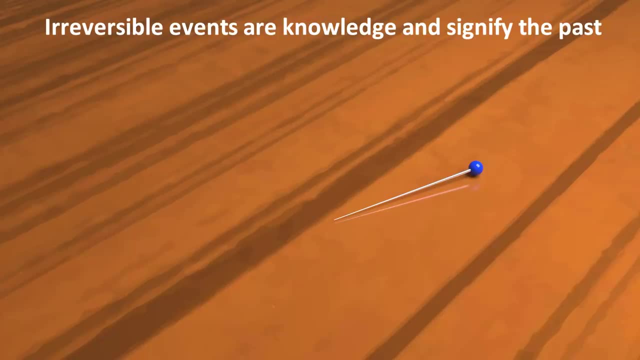 past from the present. The past, he says, is completely classical: It consists of things that definitely happened and can never unhappen. The present, though, is quantum: It's still unfolding. What seems to separate them, then, is not just whether they are reversible or not, but 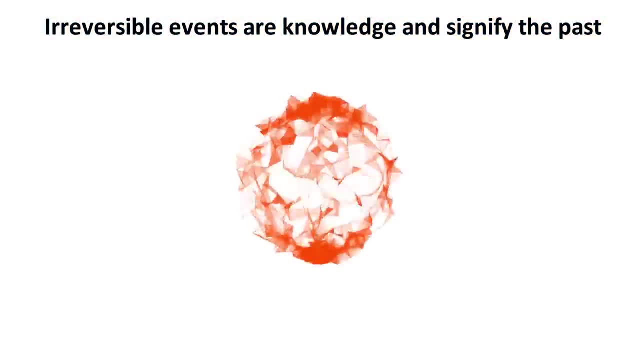 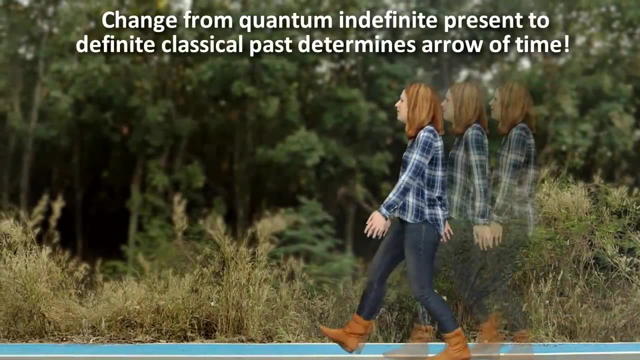 whether they are knowable or not. So what's the point of no return? What's the point of no return Whether they have become actual knowledge, something of which we can say. it was like this: According to Smolin, it's the change from a quantum indefinite present to a classical. 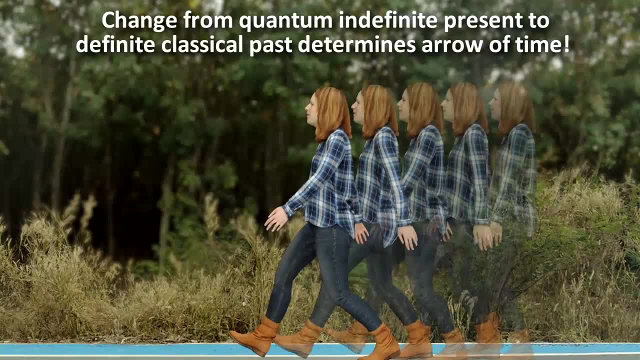 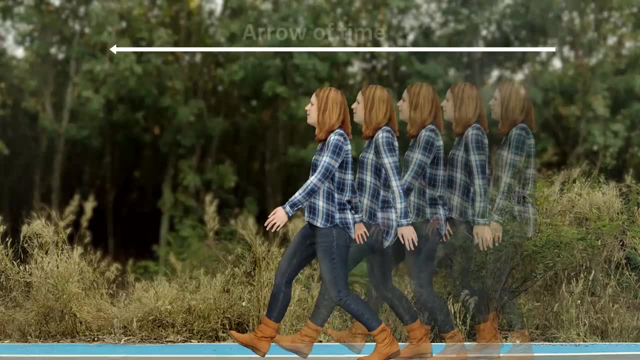 definite past that defines the very arrow of time itself, pointing it always in the forward direction, as the quantum present constantly churns out a classical past. We can never go back, We can't change the past. In fact, the past no longer really exists. 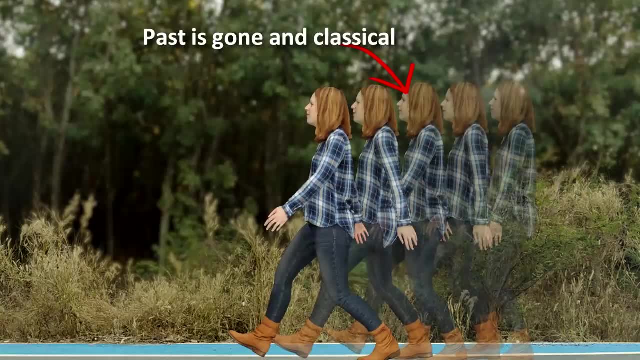 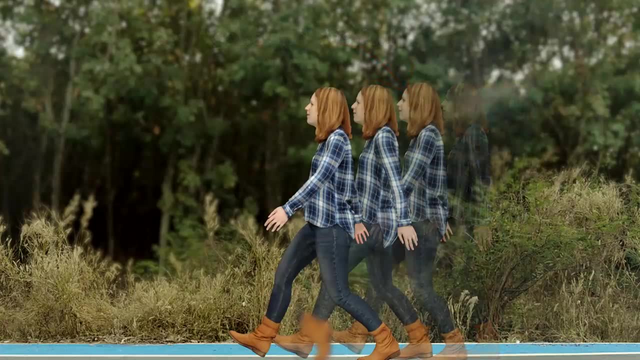 We can never go back. It doesn't really exist at all. Once something is definite, says Smolin, its job is done and it is gone. But what about the future? The future, says Smolin, is a quantum future. 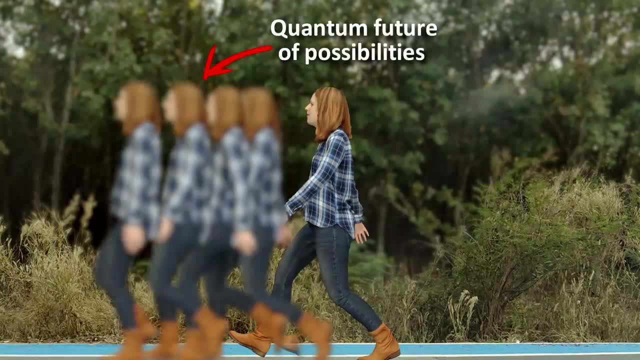 It's a place only of possibilities, not certainties. Not everything is possible in the future, though, but only things that can emerge from the present through the laws of quantum mechanics. Like the past, it doesn't truly exist, but for a different reason. 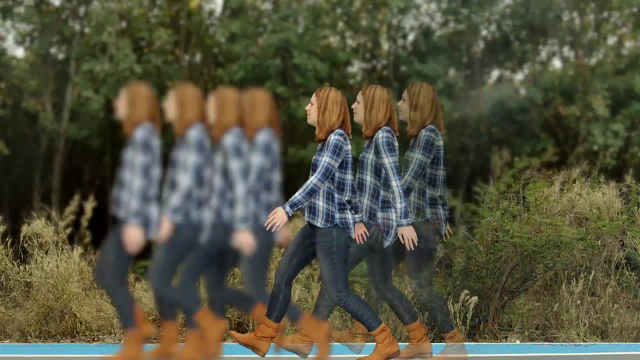 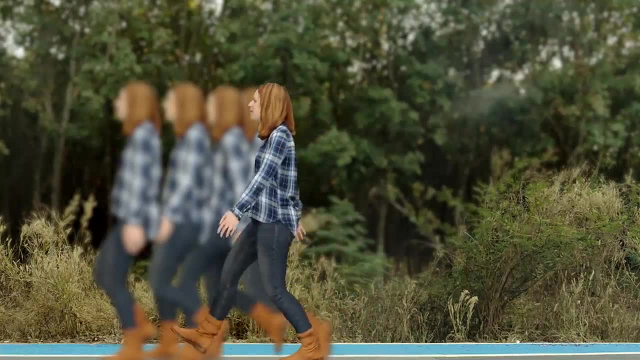 The past is not really a future. The past is not real because its job is done and it can have no further influence in the world. The future is not real because nothing in it can be made concrete until the present, forever moving forward in time, reaches it. 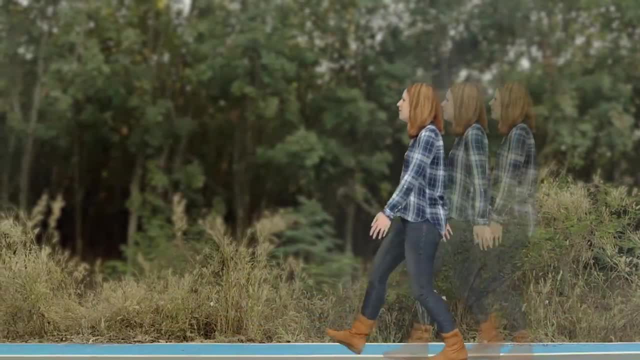 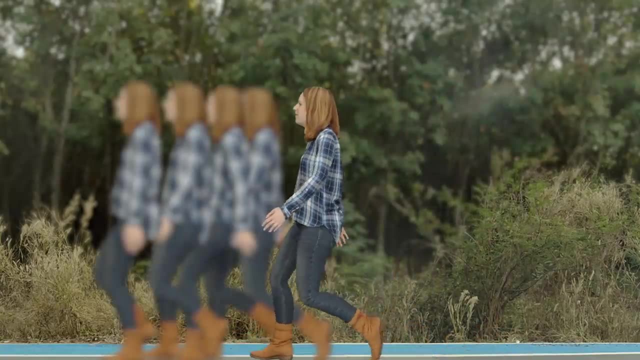 In this view, we live constantly in the moment in which probabilities are becoming actualities, in which reality- what is what has happened and what's been imprinted in the world- is at the point of condensing, Of changing from quantum to classical. 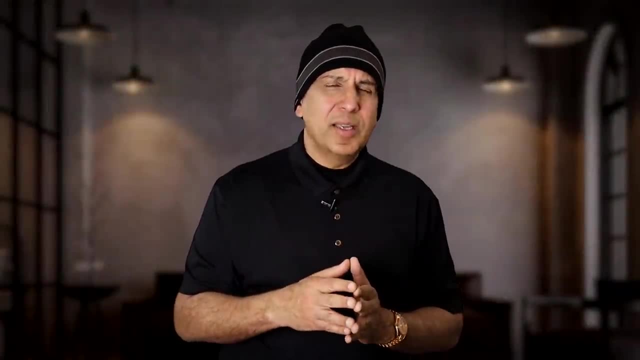 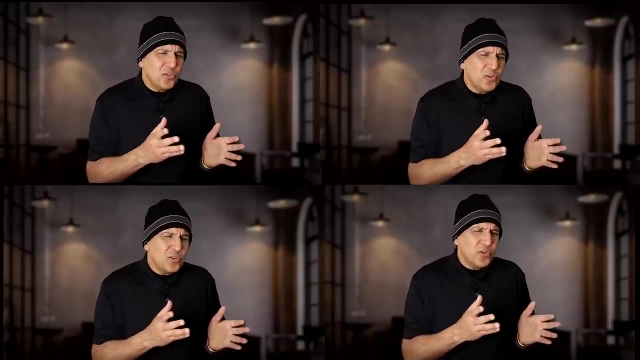 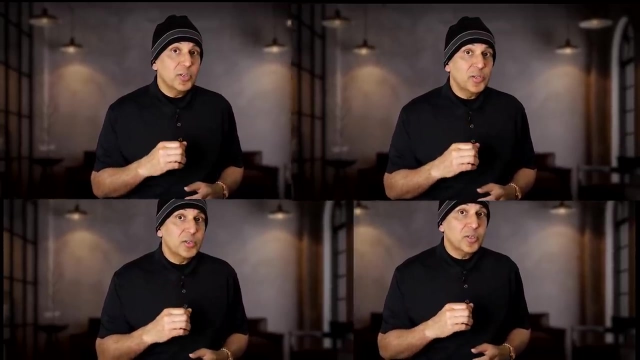 We live in the borderland. But if the future is quantum, then what happens to all those futures that aren't selected by the de-cohering present? Where do those alternative possible futures go? Do they as something, pop up in an alternative universe? 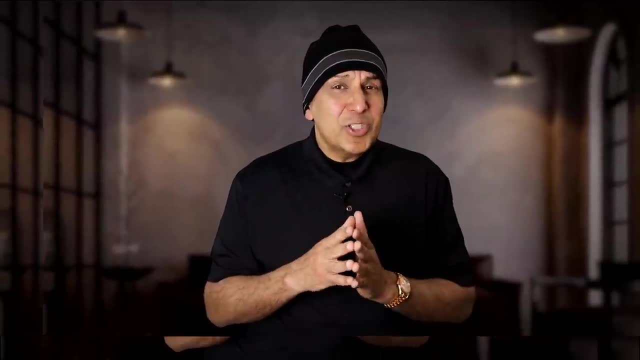 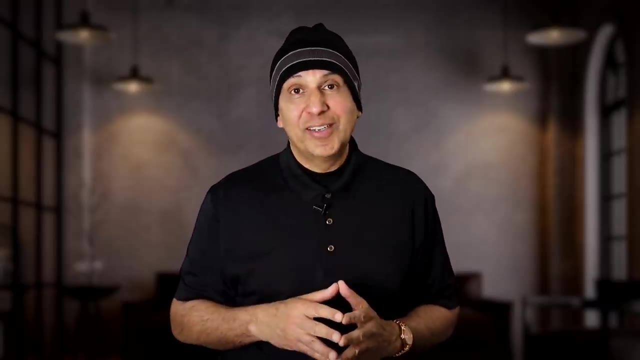 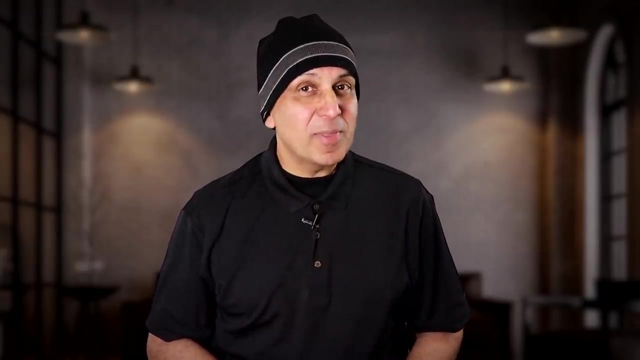 Or should we trust what our intuition seems to tell us loud and clear, that there is only one reality? That's a question no one can answer. Yet If this subject fascinates you, like it does me, and you want to learn it more in depth, 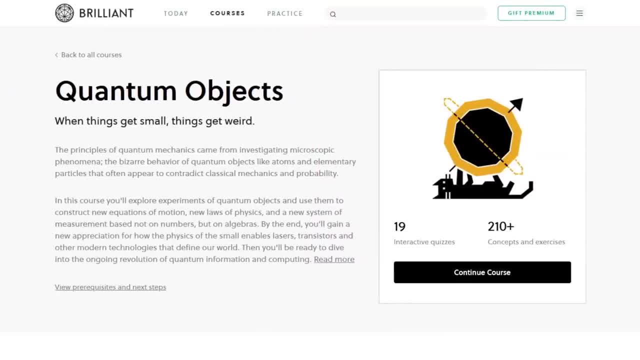 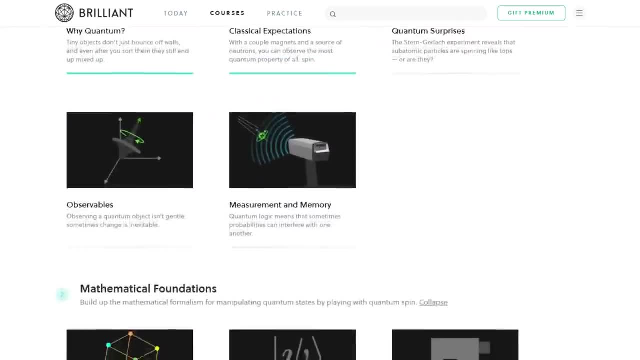 then one of the best intuitive courses offered is at Brilliant today's sponsor, called Quantum Objects. It consists of 18 interactive lessons which take you step by step through the fundamentals of quantum mechanics, including a lesson on the famous Schrodinger equation, which contains 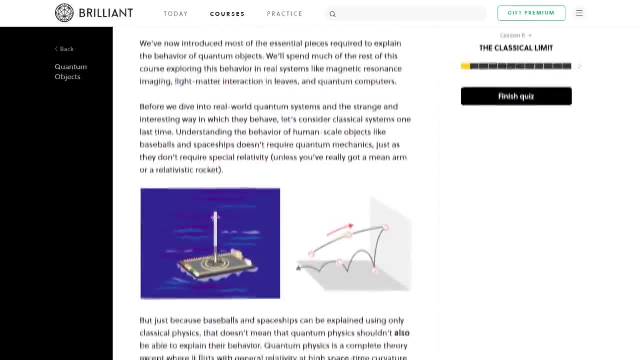 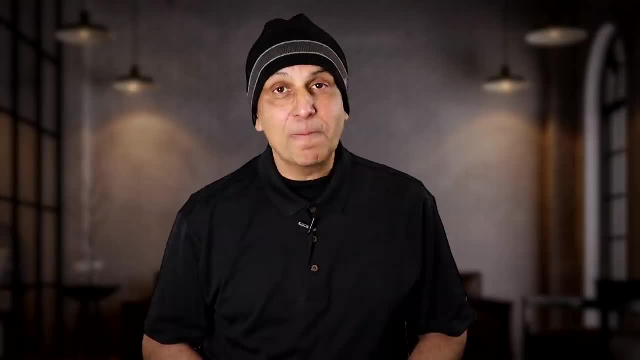 the wave function. Along the way, you'll take quizzes and solve problems. If you want to learn more about quantum mechanics, then check out our website at wwwquantumobjectscom. If you're among the first 200 people to click the link in the description, you'll get 20%. 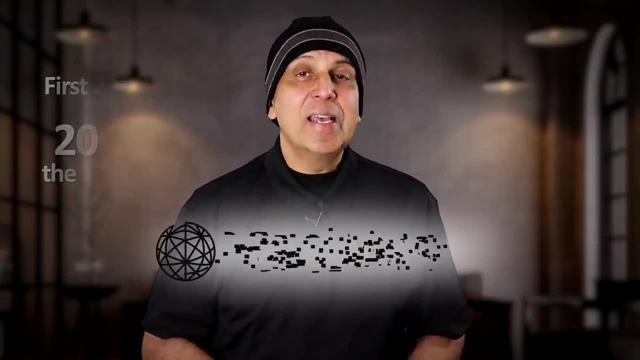 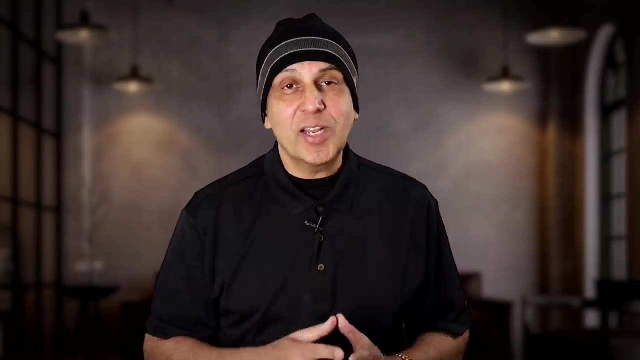 off your subscription If you haven't tried Brilliant already. this is a great opportunity to start, so be sure to click the link in the description, And if you have a question on anything you saw in this video, please feel free to leave it in the comments and I will do my very best to answer it.